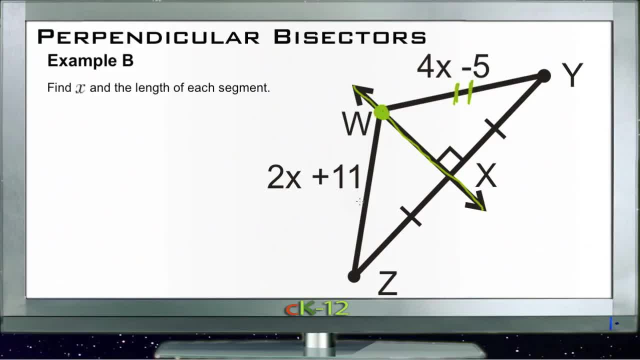 So this is going to be equidistant from Y and from Z, So those two lines are going to be the same, And that tells us that 4X minus 5 is the same thing as 2X plus 11.. So now we 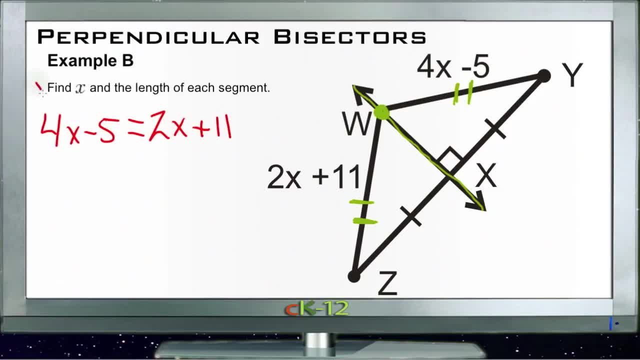 can just solve for X. So since we have more X's on this side over here, to start with let's put the X's on that side, So we'll subtract 2X over here. And since we have more X's on 2X over here, these will cancel And we'll end up with 4X minus 2X, which is 2X minus. 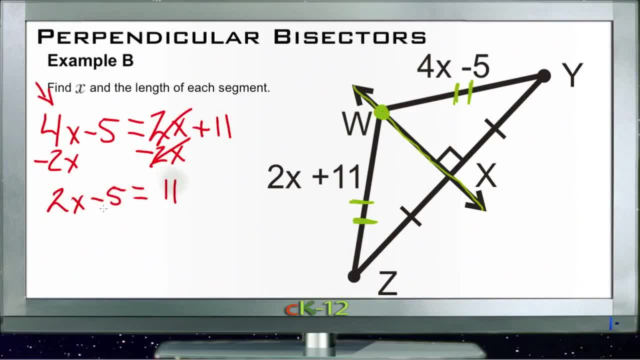 5 equals 11. And then we'll add 5 over here And similarly, and negative 5 and positive 5 make 0.. 2X equals 16. And then divide both sides by 2.. The 2's will cancel and we'll. 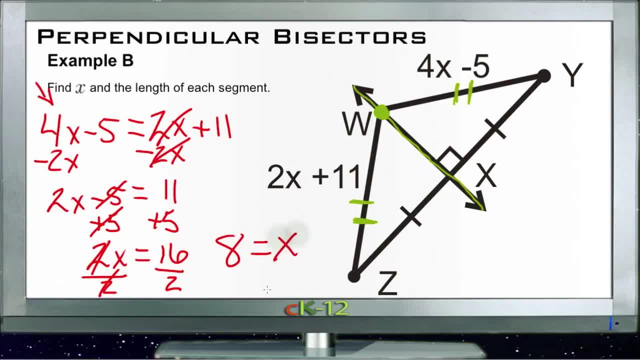 end up with: X equals 11. 8.. Sorry, I said that backwards from the way I wrote it, but X and 8 are the same thing. So if X and 8 are the same thing, then here we have 4 times 8 minus 5.. 8 times 4 is 32.. 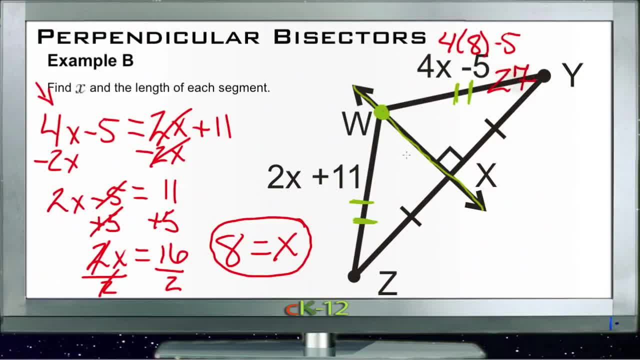 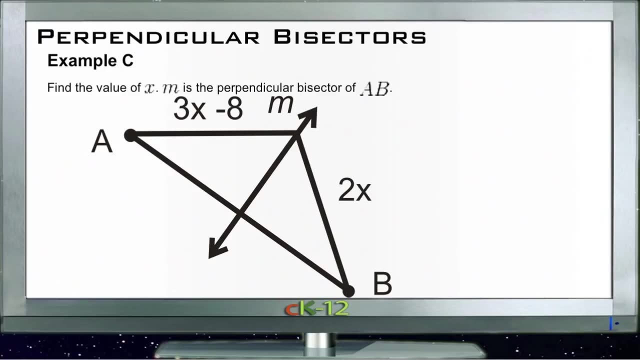 Minus 5 is 27. And 2 times 8 is 16.. Plus 11 is 27.. So X equals 8, and our two lines are 27 units. Now let's take a look at example C. Example C says: find the value of X where M is the. 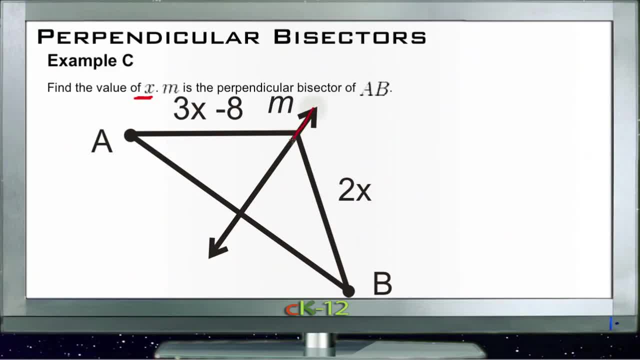 perpendicular bisector of AB. So this one is similar to the last one. We have our perpendicular bisector here And it tells us that A is the same distance from here M. I don't know if that's point A or not. We'll call that point C. A is the same distance from C as 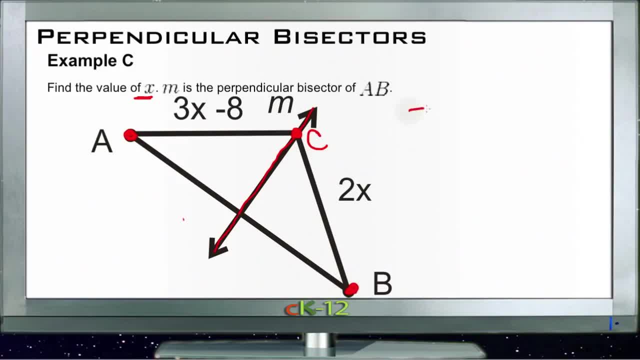 C is from B, So kind of like the last one we have: 3X minus 8 is equal to 2X, And we have more X's on this side to start with, So I'll move the X's over there. Subtract.